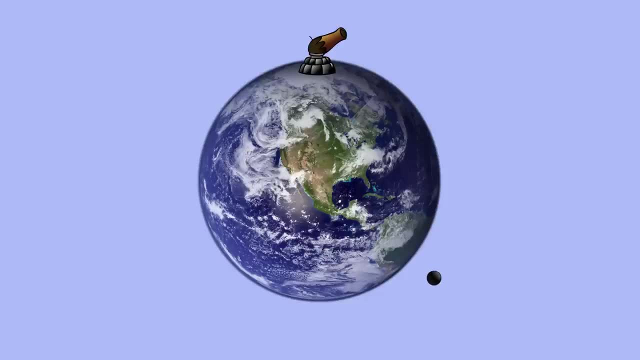 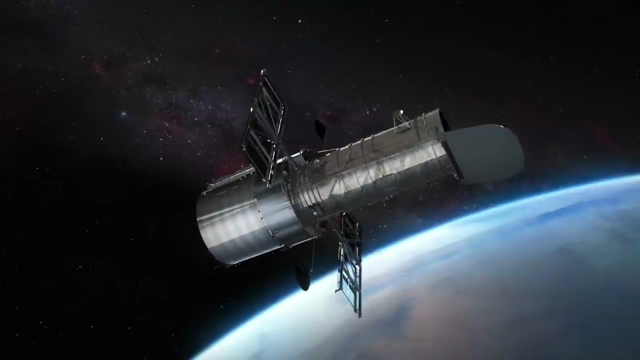 that the ball would never hit the ground, since it would fall at the same rate that earth's curvature is produced. It would thus always be falling towards the earth but never hitting it. Such an object would be said to be in orbit around the earth. Of course, no cannon can do this. 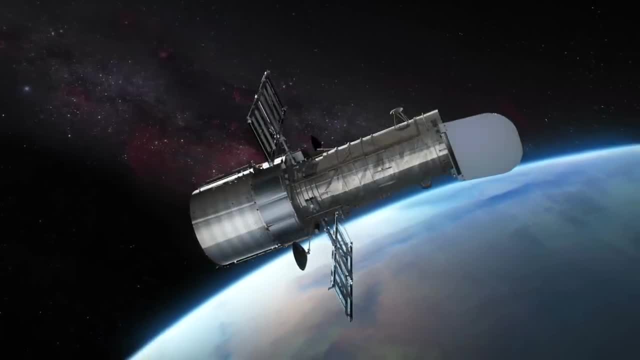 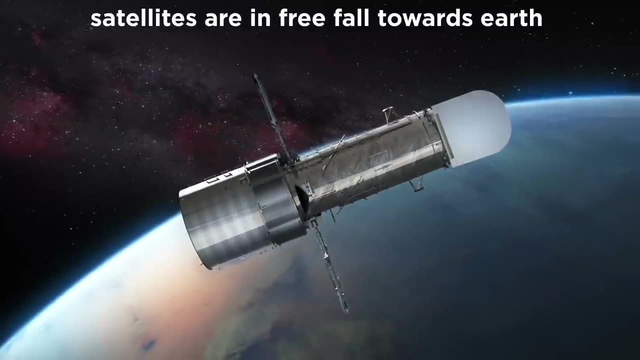 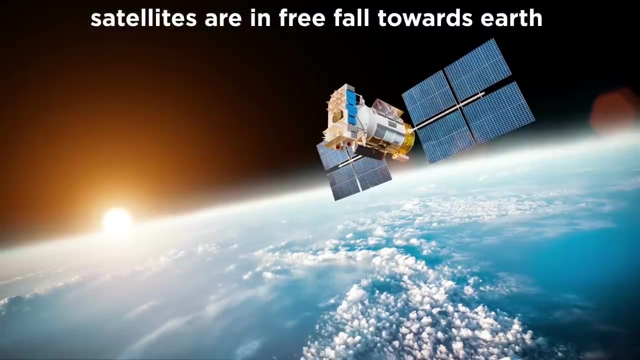 but we have finally achieved this feat with all of our satellites and space stations, which are brought up to orbit on rockets. These are very far from earth's surface and they are moving with such great speed that they, along with anyone on board, are always falling towards the earth, but never hitting it. 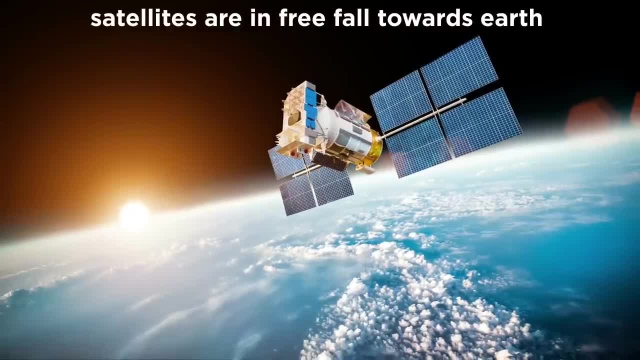 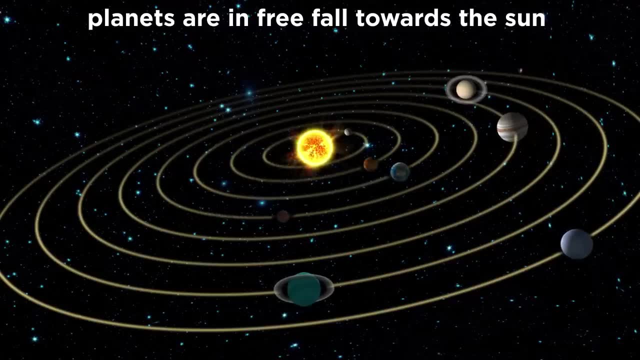 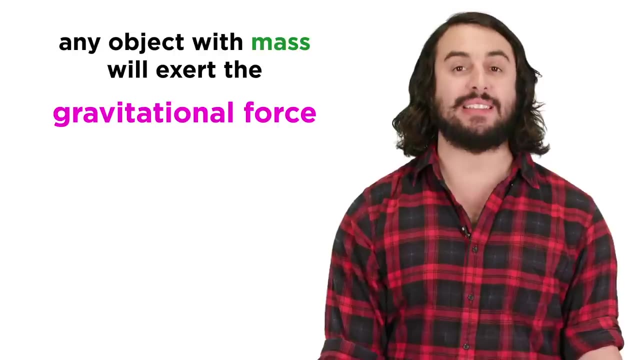 In a free fall, just like Newton's apple. This means they orbit around the earth indefinitely at a fixed speed and radius. The same can be said for all the planets around the sun. This gravitational force can describe the motion of every object in space, and it is the case that 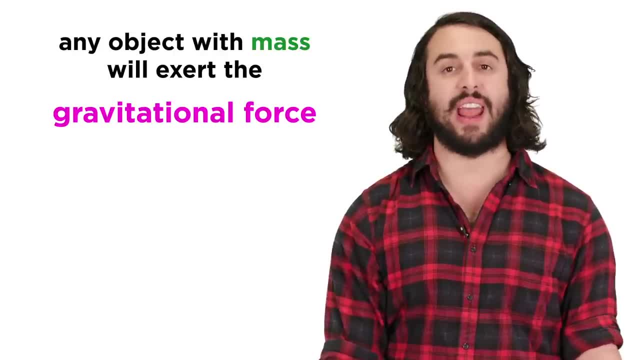 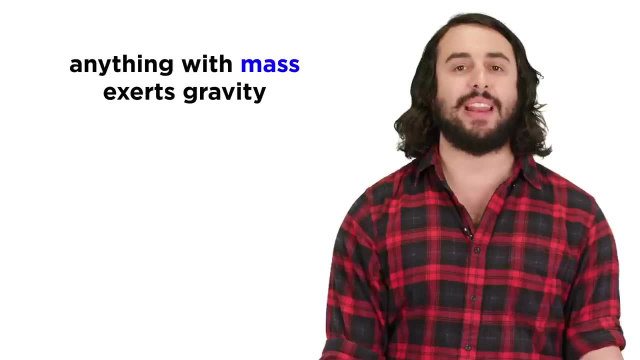 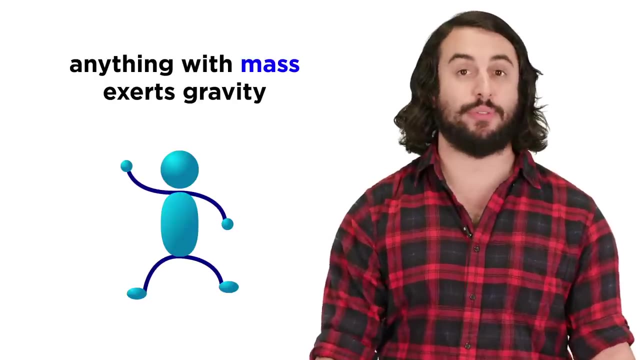 every object that contains mass will exert gravity on every other massive object. Of course, to feel the effects of gravity we must be near an enormous object like a planet. but it is completely accurate to say that gravitational force is exerted by your car, your refrigerator, even you yourself. 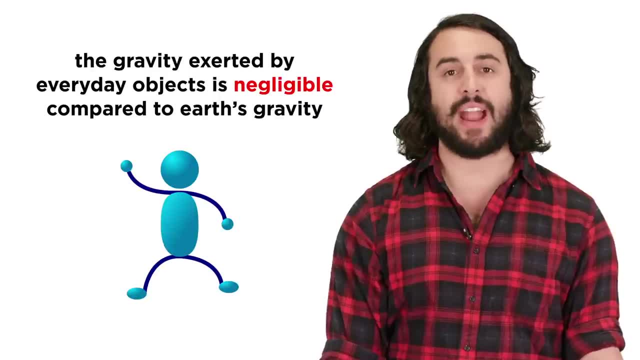 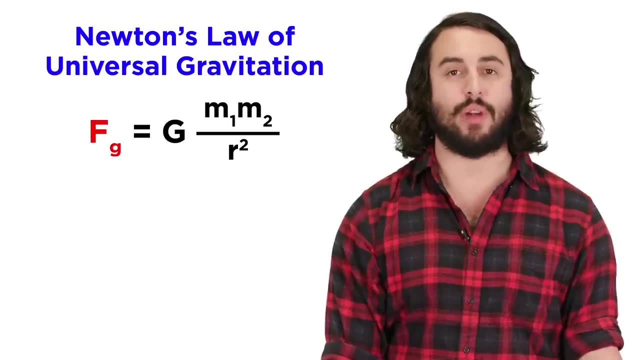 It is just that this force is completely negligible compared to the gravitational force exerted by the earth. Newton developed an equation to quantify the magnitude of the gravitational force between two objects, and it looks like this: where F is equal to the constant of universal. 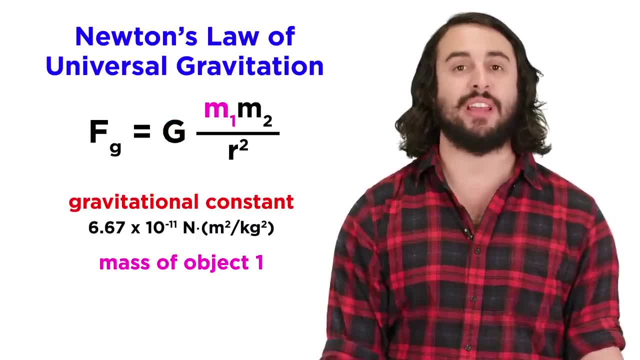 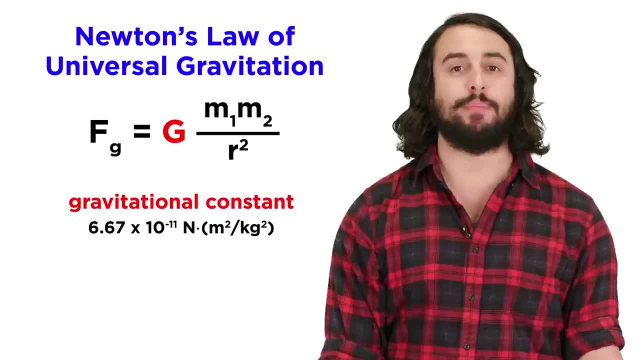 gravitation, g times the mass of the first object times the mass of the second object divided by the distance between them squared, This constant, like any other constant, simply exists so that a natural phenomenon like gravity can be expressed in our own arbitrary, man-made units, and it is. 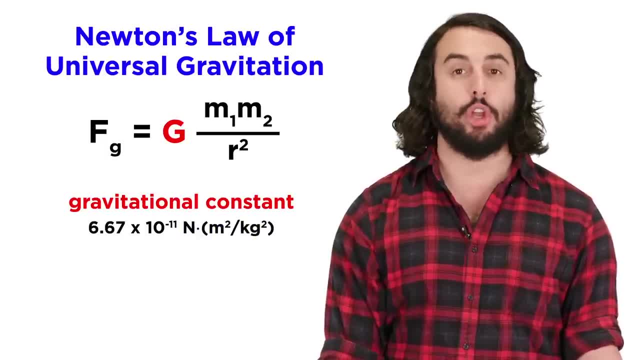 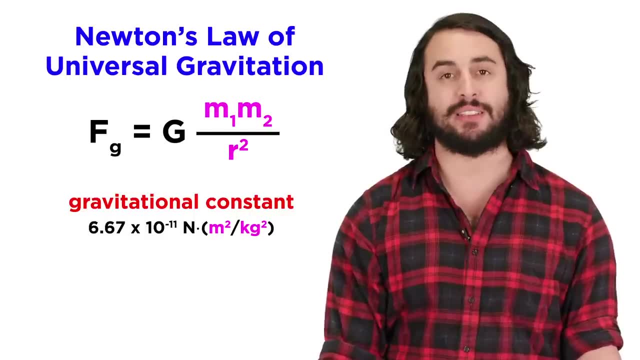 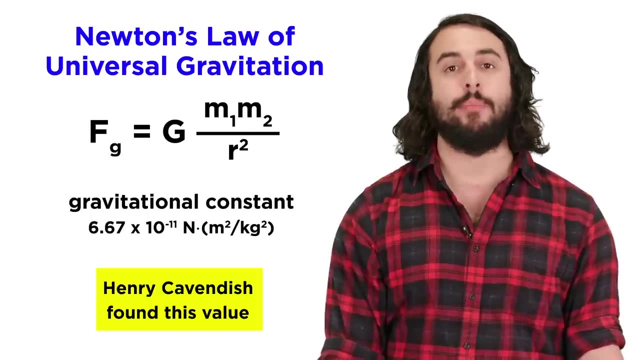 equal to 6.67 times ten, to the negative eleven Newton meters squared over kilograms squared. These are the units that will cancel out the units on the masses and radius so as to give a value for force in Newtons. This value was not known to Newton at the time, but was determined experimentally. 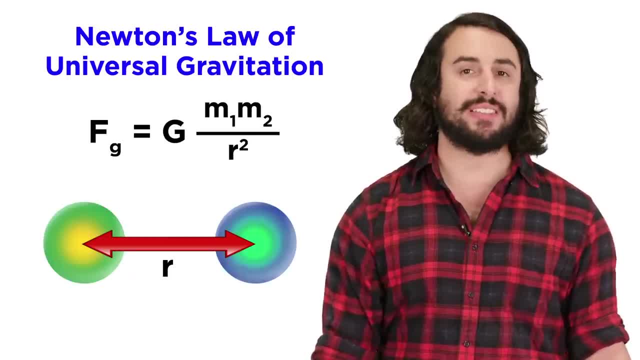 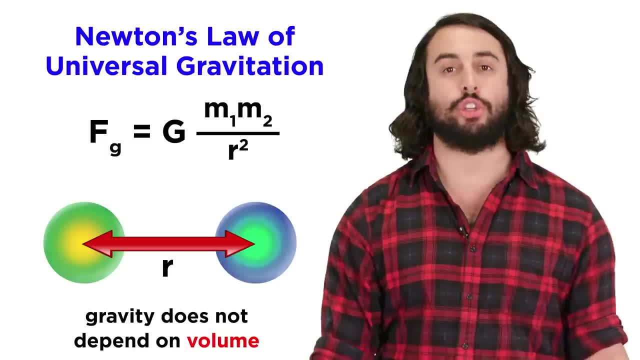 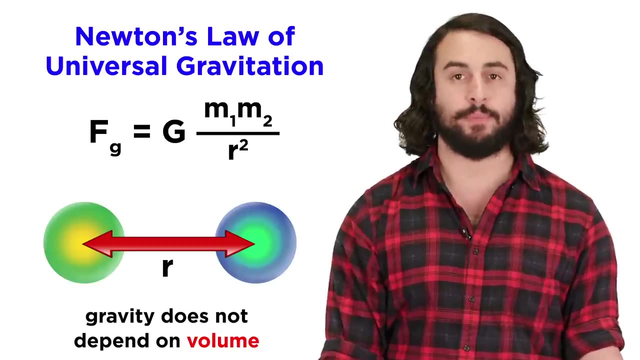 about a hundred years later by Henry Cavendish. When discussing the radius between two objects, we will take the distance between their centers rather than their surfaces, as Newton showed that the gravitational force exerted by an object depends only on its mass and not on its volume. 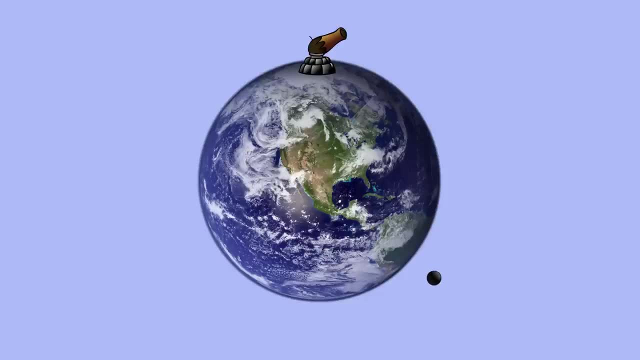 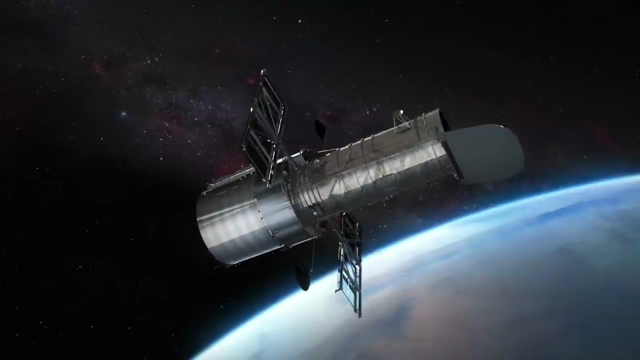 that the ball would never hit the ground, since it would fall at the same rate that earth's curvature is produced. It would thus always be falling towards the earth but never hitting it. Such an object would be said to be in orbit around the earth. Of course, no cannon can do this. 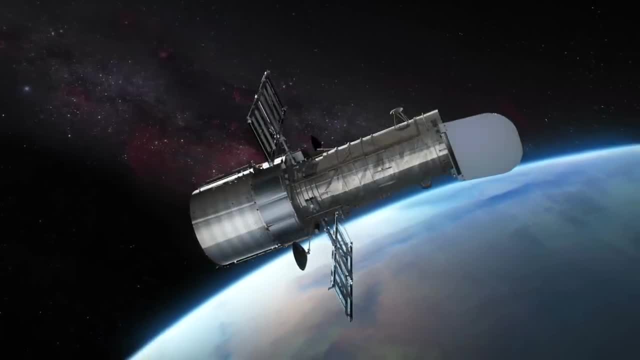 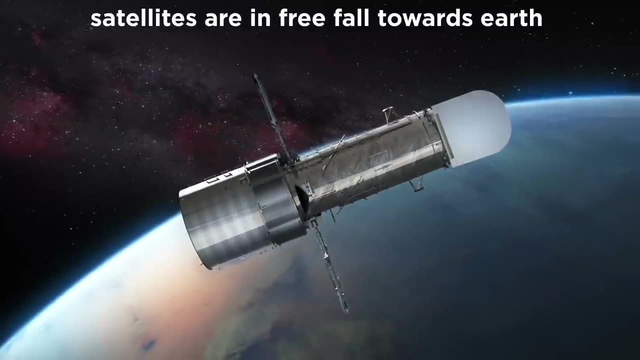 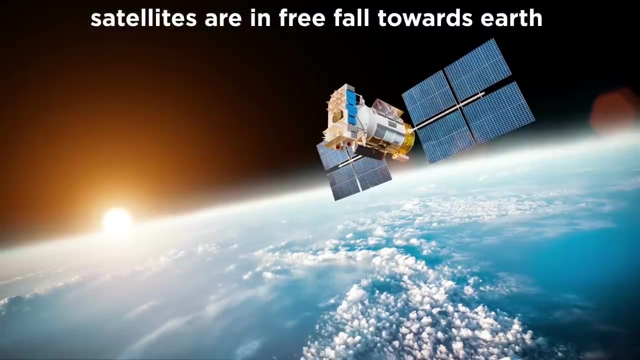 but we have finally achieved this feat with all of our satellites and space stations, which are brought up to orbit on rockets. These are very far from earth's surface and they are moving with such great speed that they, along with anyone on board, are always falling towards the earth, but never hitting it. 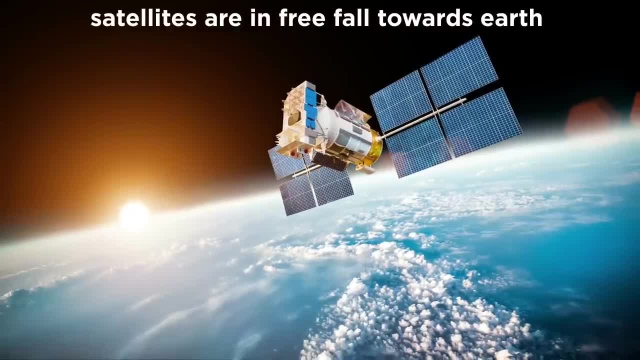 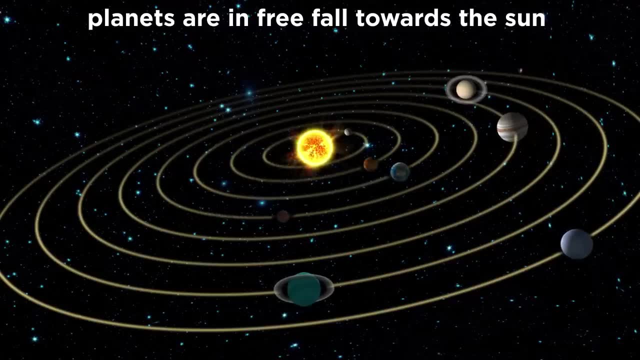 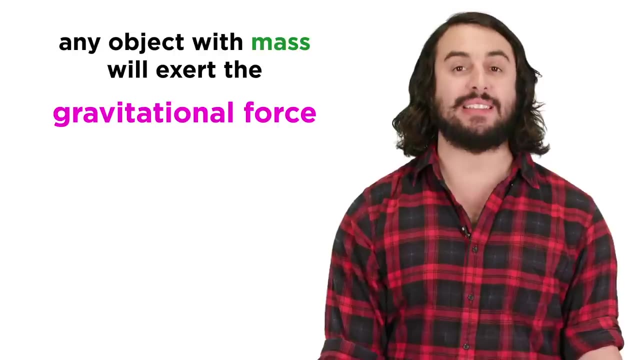 In a free fall, just like Newton's apple. This means they orbit around the earth indefinitely at a fixed speed and radius. The same can be said for all the planets around the sun. This gravitational force can describe the motion of every object in space, and it is the case that 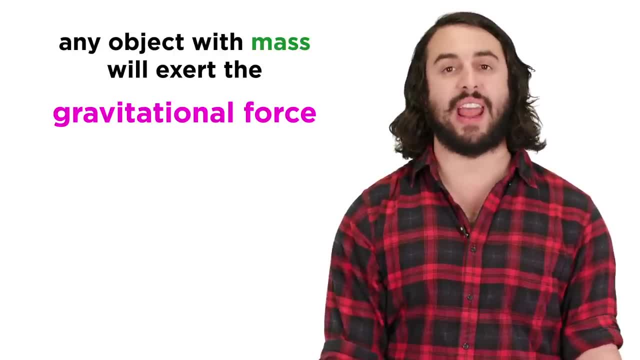 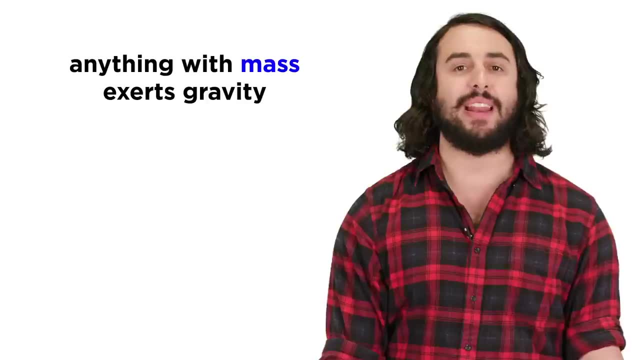 every object that contains mass will exert gravity on every other massive object. Of course, to feel the effects of gravity we must be near an enormous object like a planet. but it is completely accurate to say that gravitational force is exerted by your car, your refrigerator, even you yourself. 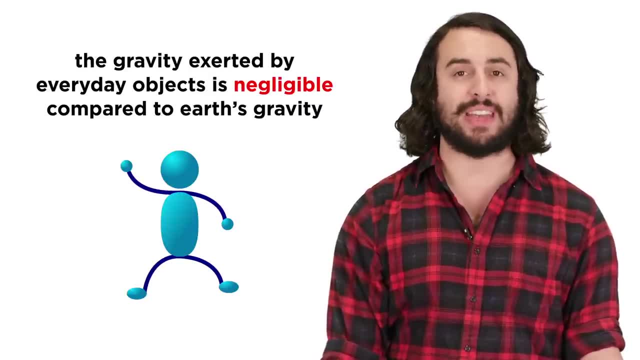 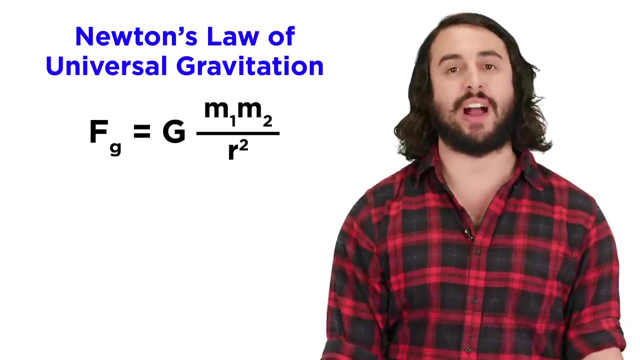 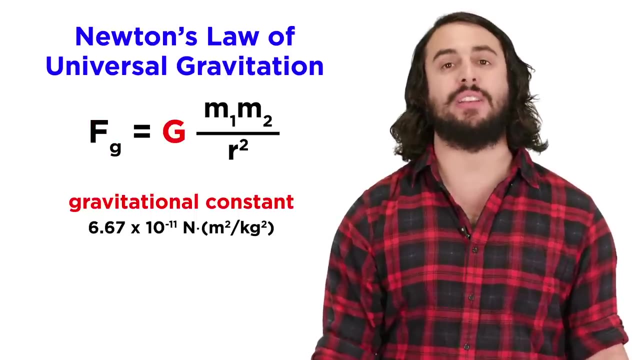 It is just that this force is completely negligible compared to the gravitational force exerted by the earth. Newton developed an equation to quantify the magnitude of the gravitational force between two objects, and it looks like this: where F is equal to the constant of universal gravitation, G, 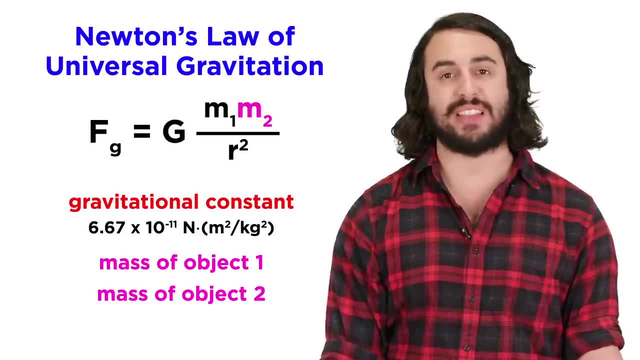 times the mass of the first object, times the mass of the second object, divided by the distance between them squared, This constant, like any other constant, simply exists so that a natural phenomenon like gravity can be expressed in our own arbitrary, man-made units, and it is equal. 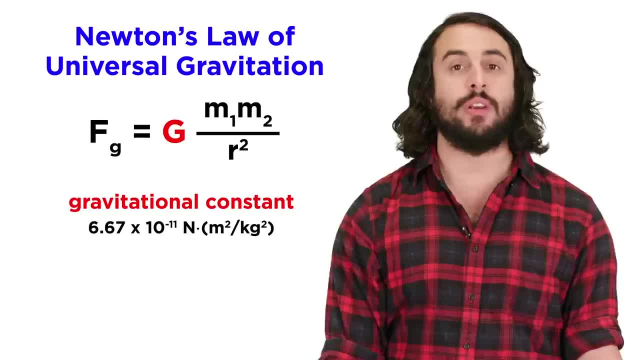 to 6.67 times 10 to the negative 11 Newton meters squared over kilograms squared. These are the units that will cancel out the units on the masses and radius so as to give a value for force in Newtons. This value was not known to. 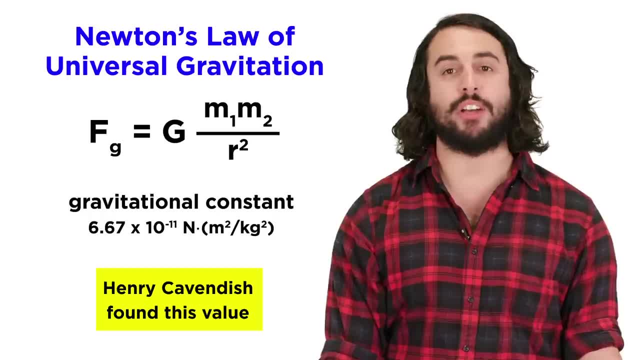 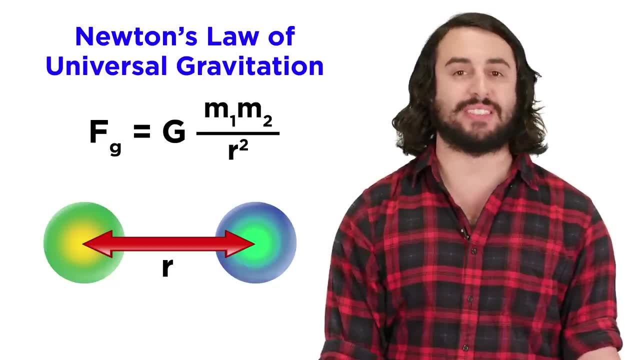 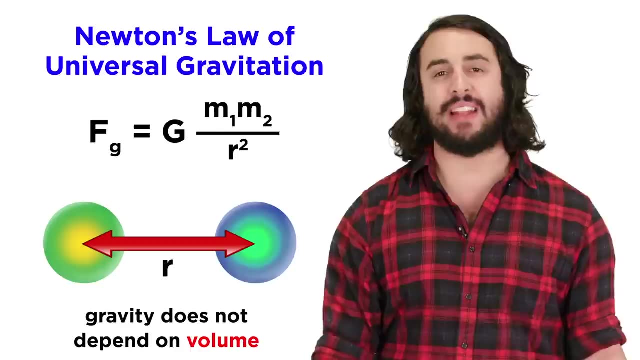 Newton at the time, but was determined experimentally about a hundred years later by Henry Cavendish. When discussing the radius between two objects, we will take the distance between their centers rather than their surfaces, as Newton showed that the gravitational force exerted by an object depends only on its 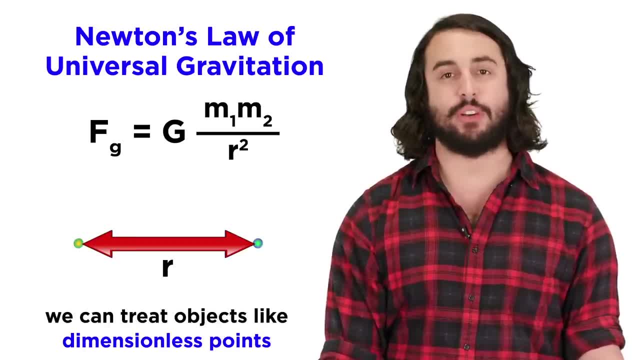 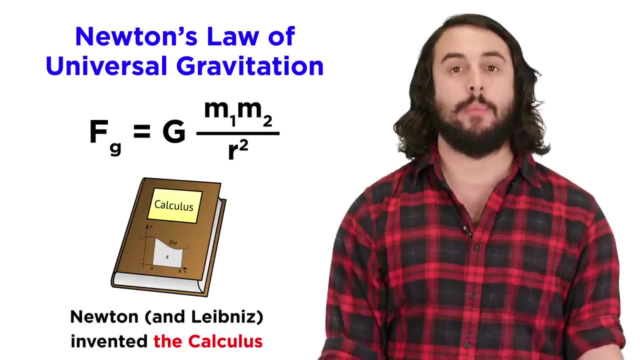 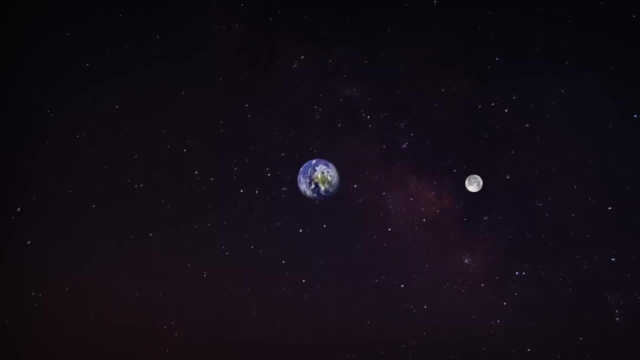 mass and not on its volume, meaning that when discussing gravity, we can treat everything as a point-like mass. He had to invent the calculus to do so, much to the dismay of math students everywhere you. When examining a system like the Earth and the Moon, we must understand that. 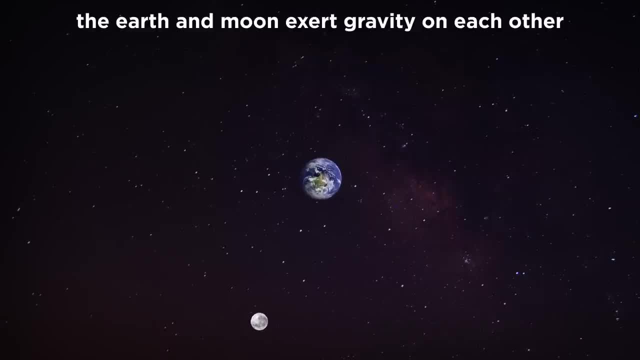 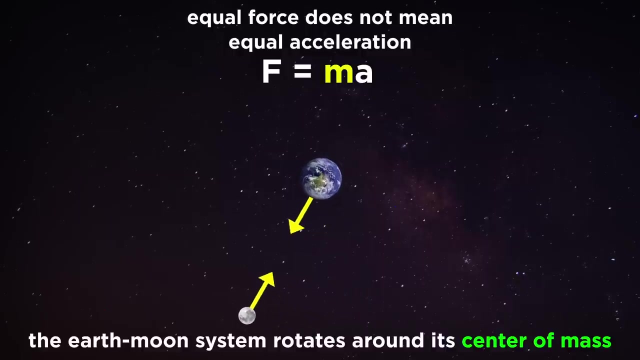 both of these objects exert gravitational force on the other and that these forces are equal in magnitude, meaning that both of these bodies rotate around their combined center of mass. But don't forget that F equals ma, so equal forces will not produce equal accelerations if the masses are. 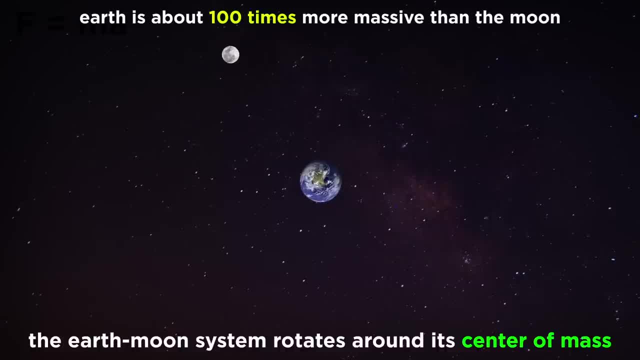 different. As it happens, the Earth is much, much more massive than the Moon, so the mutual gravitational force is able to accelerate the Moon more than the Earth, and the center of mass for the system lies within the Earth itself, which is why we simply observe. 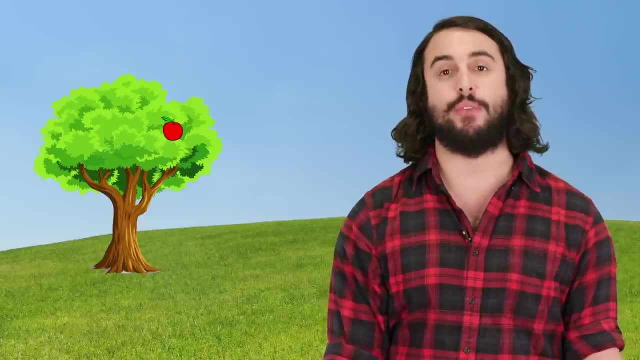 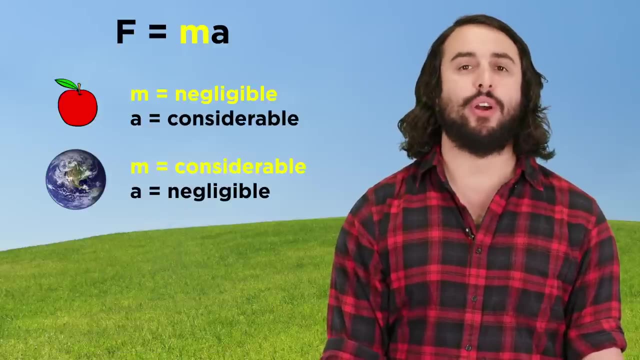 the Moon going around the Earth. The same can be said for Newton's falling apple. The apple accelerates towards the Earth and the Earth accelerates towards the apple. but the Earth is more massive than the apple by an inconceivable factor. so 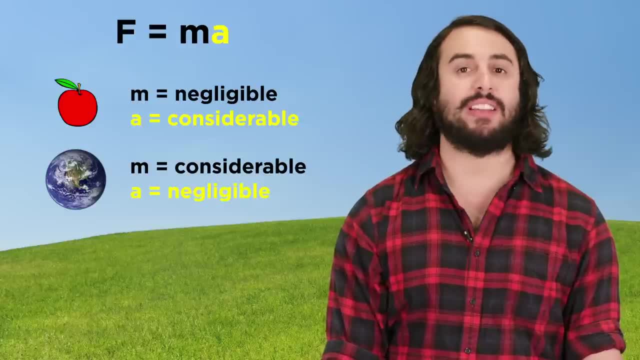 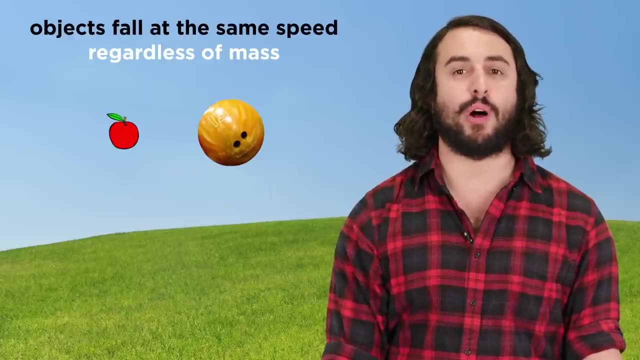 the acceleration of the Earth is not even measurable, whereas we can visually confirm the acceleration of the apple. Furthermore, we want to understand that an apple will fall to the Earth with the same acceleration as a bowling ball or any other massive object if we disregard. 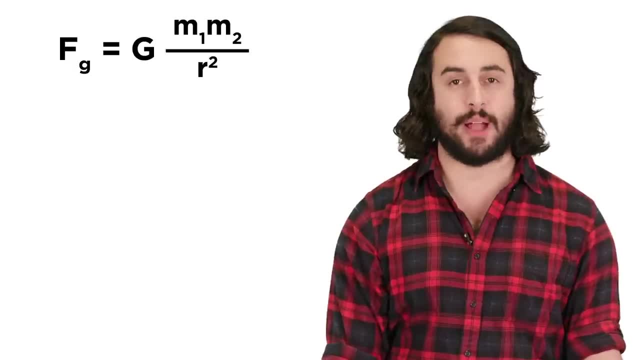 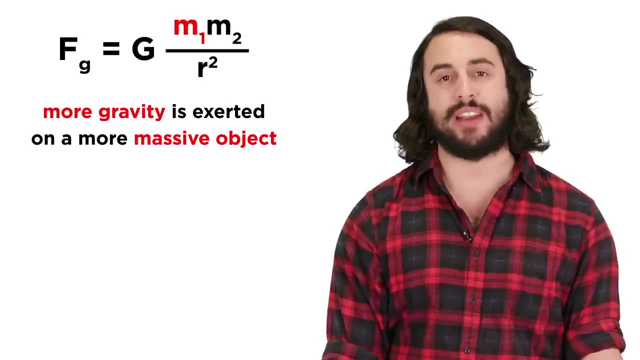 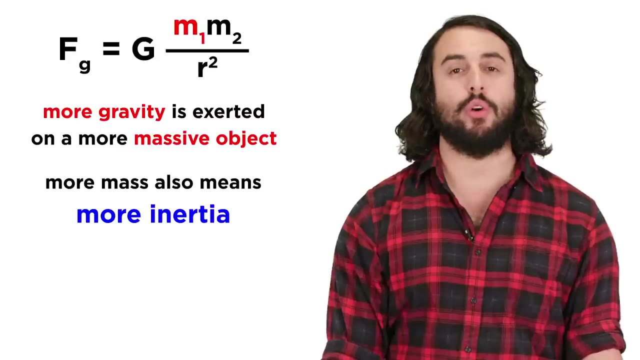 wind resistance. Although counterintuitive to some, we can rationalize this if we understand that while the force of gravity is able to impart greater acceleration on a more massive object, the more massive object also has greater inertia resistance to being accelerated, so the 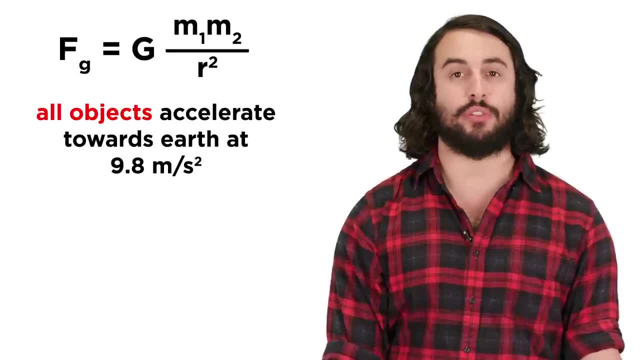 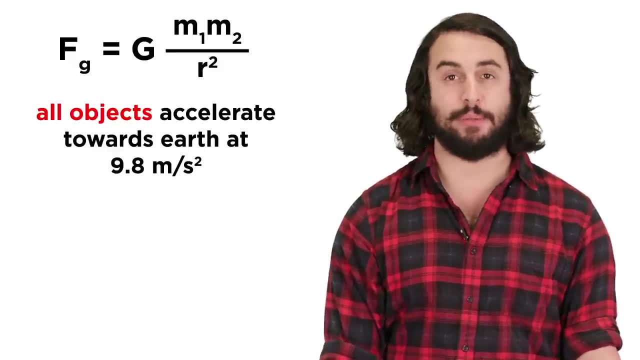 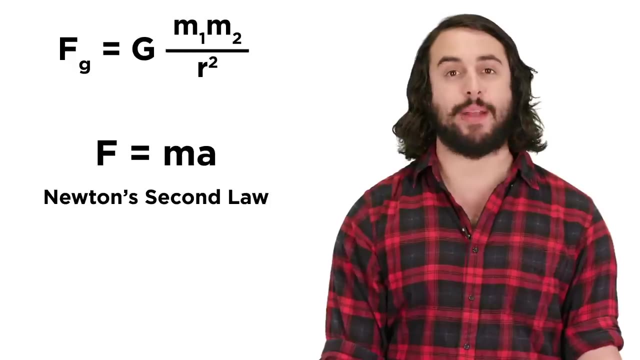 end result is that all objects accelerate towards Earth in the same way, at 9.8 meters per second squared. This fact is easy to derive if we do some algebraic manipulation. We know that a falling object exhibits behavior. according to Newton's second law, F equals ma, where 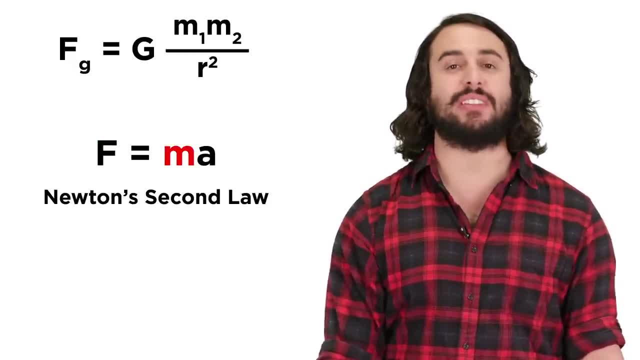 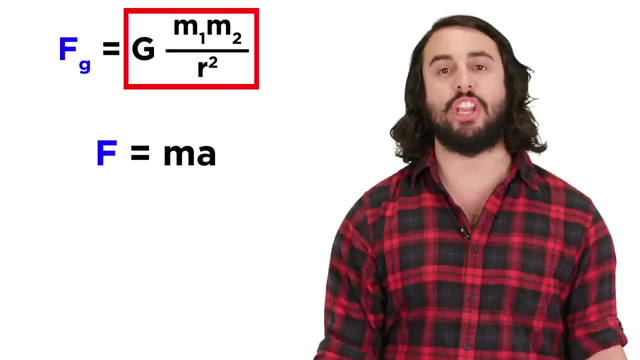 the force that generates the falling is equal to the mass of the object times its acceleration. but this force is the gravitational force. so we can also model this behavior with gm1m2 over r squared, where m1 is the mass of the object and 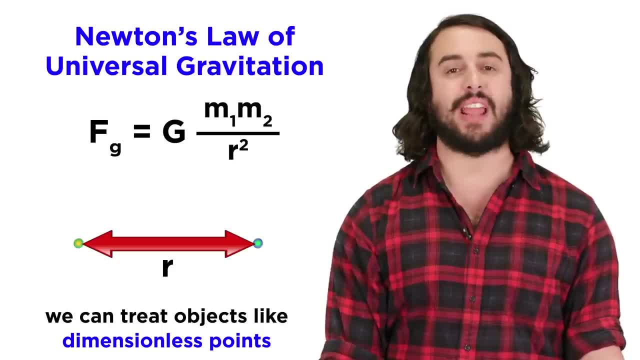 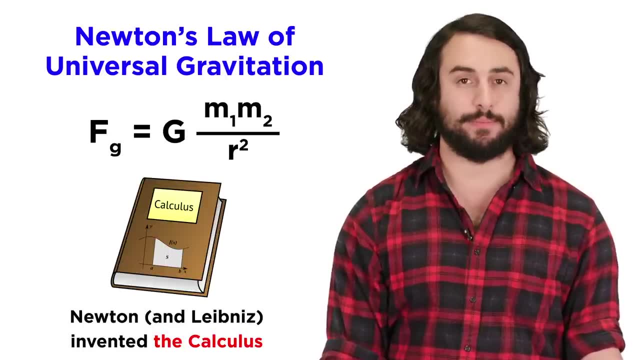 meaning that when discussing gravity, we can treat everything as a point-like mass. He had to invent the calculus to do so, much to the dismay of math students everywhere. When examining a system like the earth and the moon, we must understand that both of these 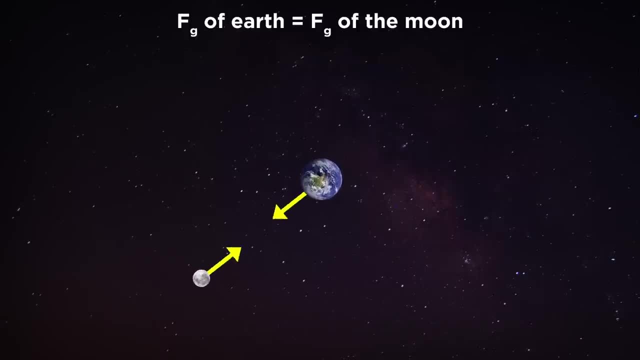 objects exert gravitational force on the other and that these forces are equal in magnitude, meaning that both of these bodies rotate around their combined center of mass. But don't forget that F equals ma, so equal forces will not produce equal accelerations if the masses 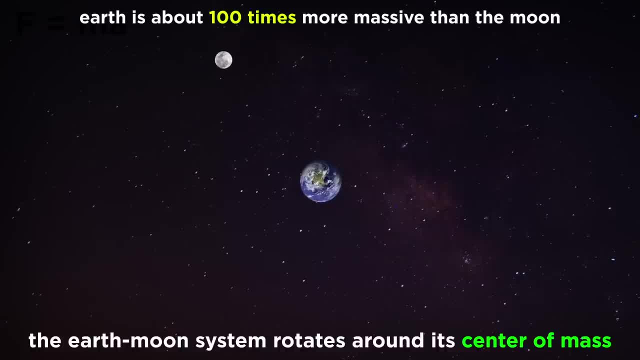 are different. As it happens, the earth is much, much more massive than the moon, so the mutual gravitational force is able to accelerate the moon more than the earth, and the center of mass for the system lies within the earth itself, which is why we simply observe the moon going around the 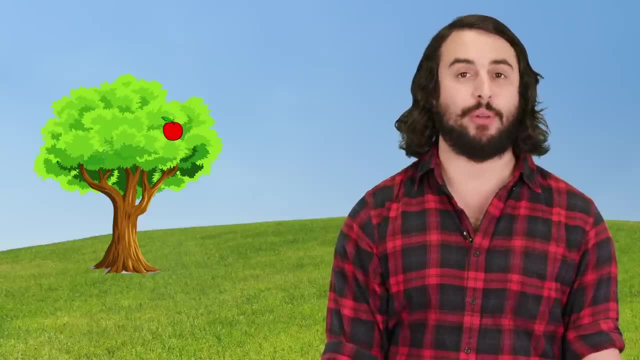 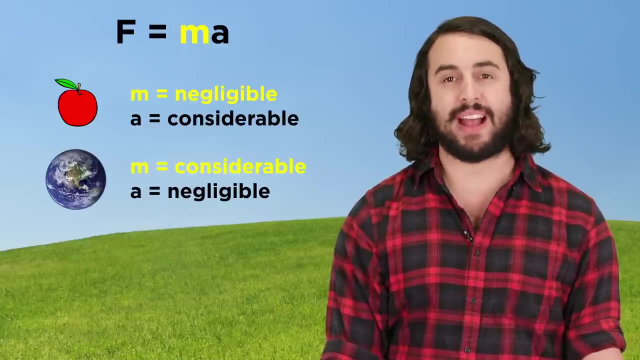 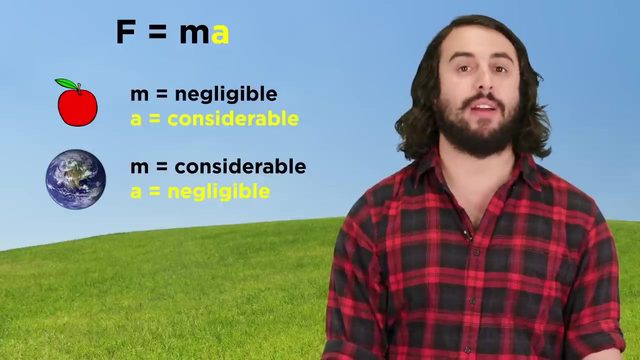 earth. The same can be said for Newton's falling apple. The apple accelerates towards the earth and the earth accelerates towards the apple. But the earth is more massive than the apple by an inconceivable factor, so the acceleration of the earth is not even measurable, whereas we can. 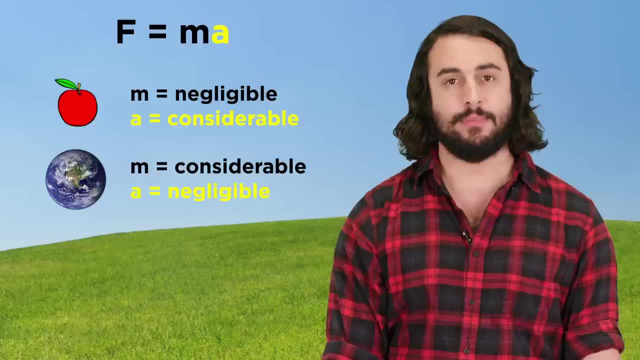 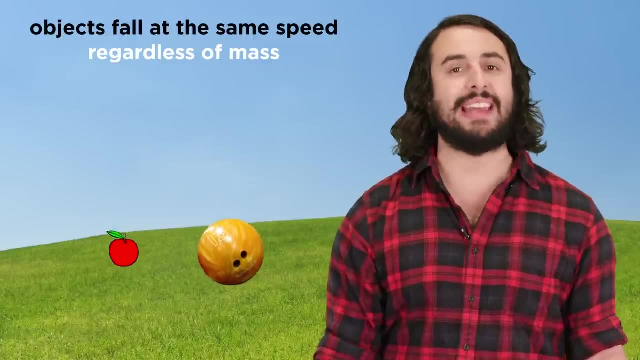 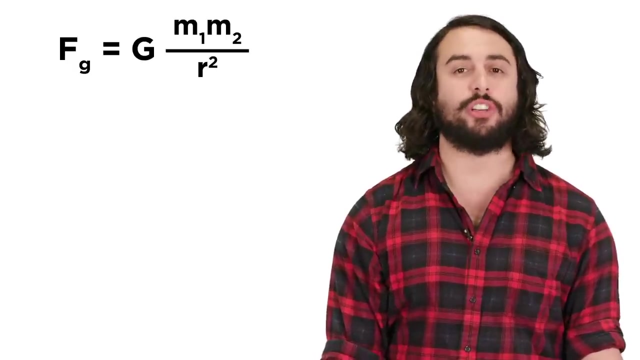 visually confirm the acceleration of the apple. Furthermore, we want to understand that an apple will fall to the earth with the same acceleration as a bowling ball or any other massive object, if we disregard wind resistance, Although counterintuitive to some, we can rationalize this if we understand that, while the force of gravity is able to impart, 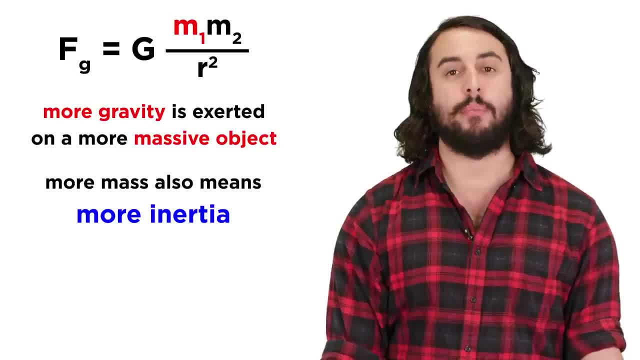 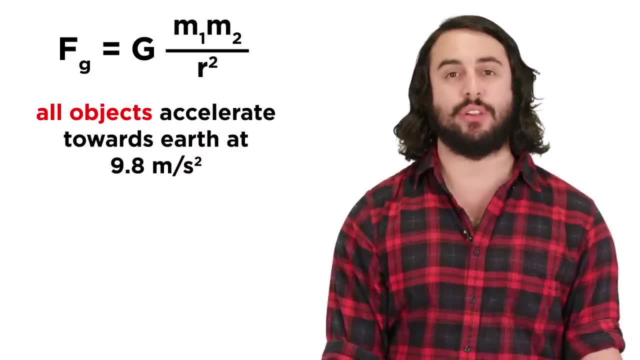 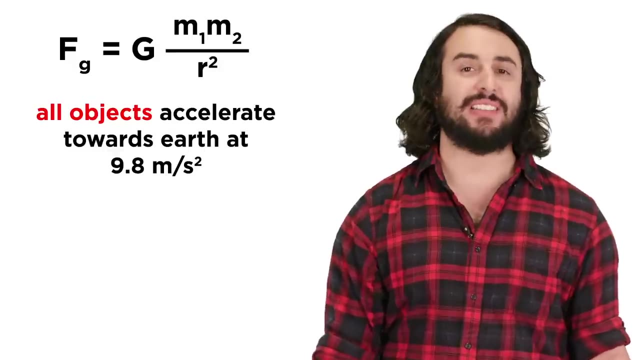 greater acceleration on a more massive object, the more massive object also has greater inertia or resistance to being accelerated. so the end result is that all objects accelerate towards earth in the same way, at 9.8 meters per second squared. This fact is easy to derive, if we do some. 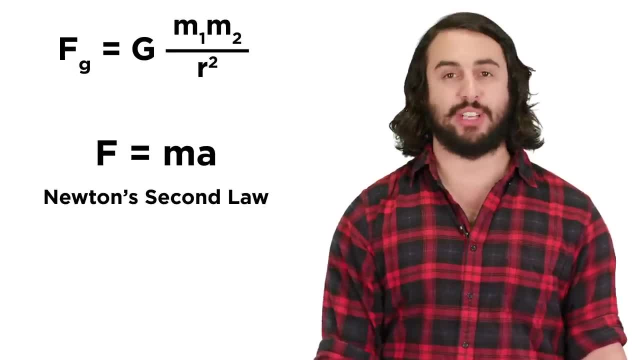 algebraic manipulation. We know that a falling object exhibits behavior. according to Newton's second law, F equals ma, where the force that generates the falling is equal to the mass of the object times its acceleration. But this force is the gravitational force, so we can also model.